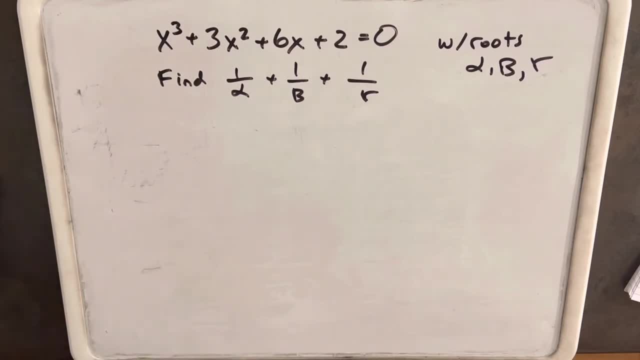 a cubic or a higher degree polynomial. So let's look at a generic. Instead of looking at the specific cubic, let's look at the generic form: ax cubed plus bx squared, plus cx plus t squared. So let's look at the generic form: ax cubed plus bx squared, plus cx plus t squared. 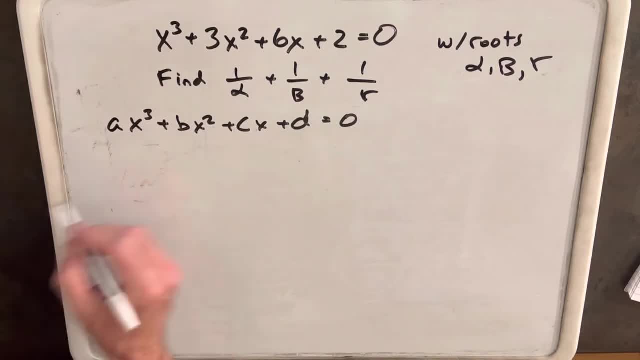 equals 0. Vieta's formula tells us that the sum of all the roots, alpha, beta, r, is just minus b over a. Then it tells us that the sum of the product of the roots by 2,, 2 at a time. 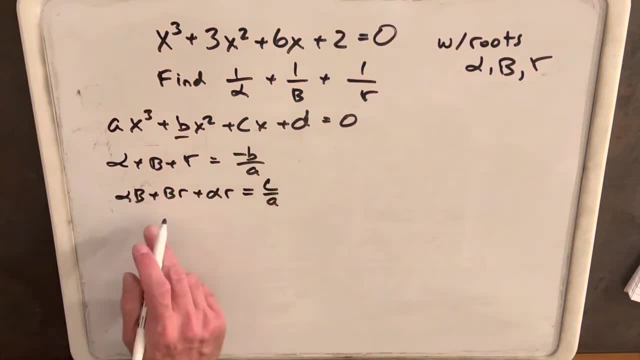 is going to be c over a, and then the product of all the roots, alpha times, beta times, r is going to be minus d over a. And so if you were doing that, a higher degree, polynomial, a fifth degree, seventh degree, whatever, it has the same pattern. 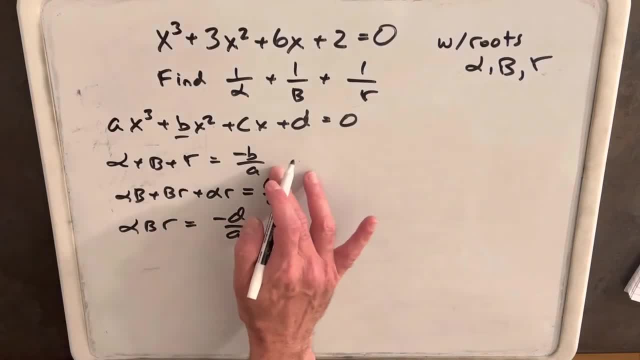 of the sum of the roots will be this minus b over a, and then by 2 will be the next one, c over a, and it'll just continue until you have the product of the roots. but it's obviously a little more messy when you have a higher degree polynomial. 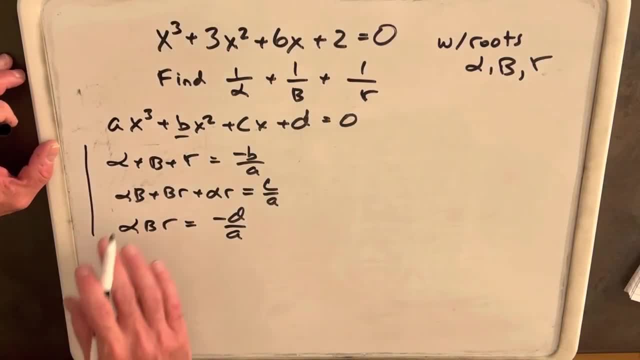 So notice that Vieta's formula gives us a way to find the sums and products of the roots by the sum of the products of the roots. So we have some useful information. but this isn't great necessarily if we have to find the roots exactly. But luckily this problem doesn't ask us to find. 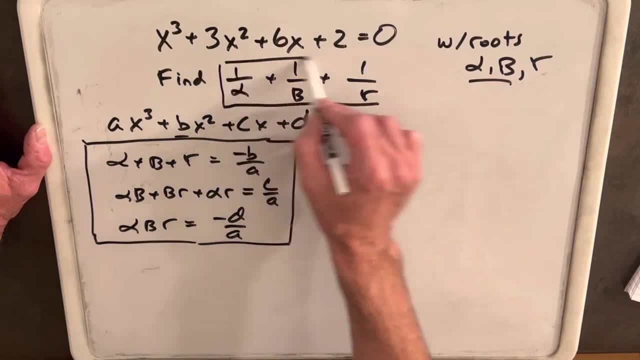 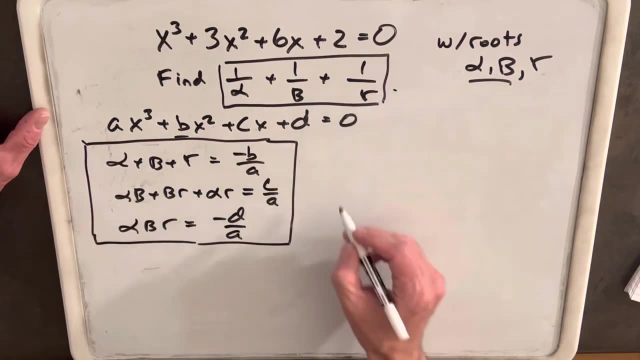 the roots. it asks us to find this, which we can simplify. Hopefully, we can then use these Vieta formulas. So let's look at this piece. What we can do here is we can get a common denominator by just multiplying, like so for a common denominator, we can get a common denominator. 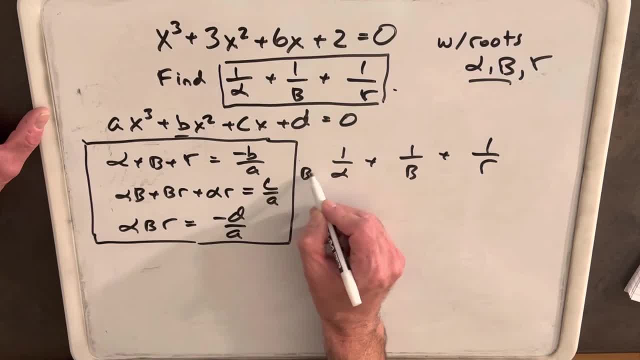 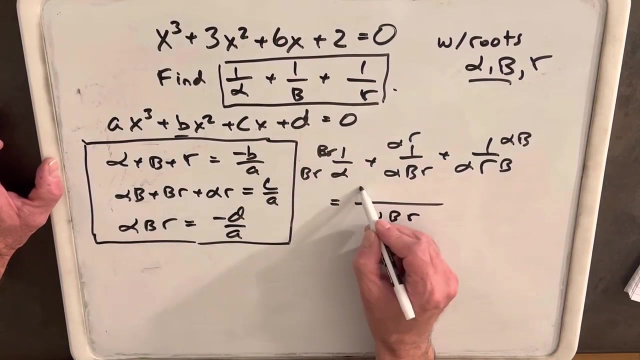 alpha will multiply times beta r on top and bottom. So we're just multiplying by 1, but we'll do the same for each of these And then. so when we add this together with our common denominator, our common denominator will be alpha beta r. it's just going to be beta r plus alpha, r plus alpha. 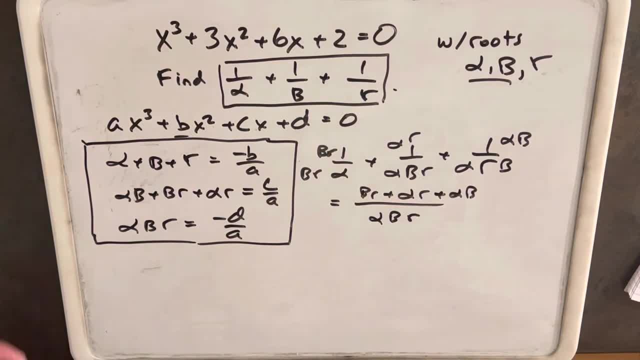 beta. And the good thing about this is our denominator is actually just the product of the roots here, And the numerator is the sum of the roots by 2, which is our value in the middle here. Then, with these formulas, we have everything we need to actually go ahead and solve this problem. 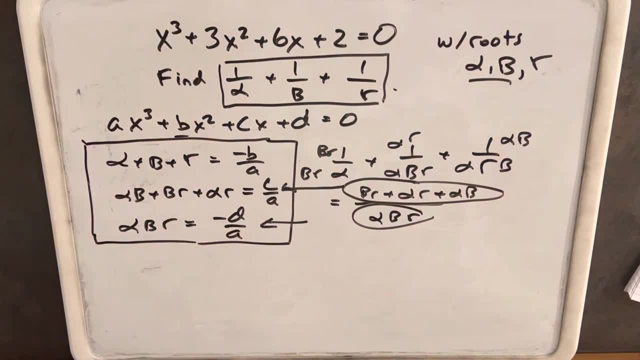 for these roots. So let's do that, And even though we don't need this first thing, we'll find that anyway. So for our problem, alpha plus beta plus our minus b value, so minus 3 over 1, which is just minus 3.. 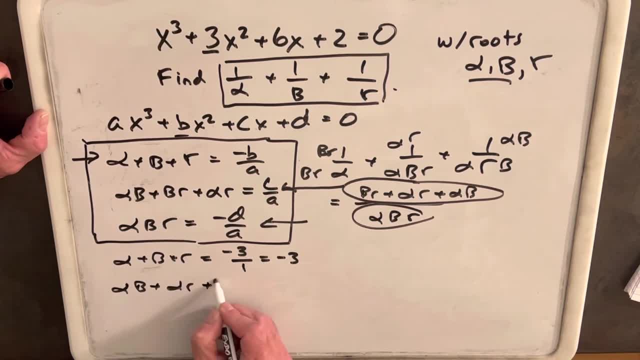 The sum of the roots, two at a time, is going to be our c value over 1.. So it's going to be 6.. And then the product of our roots is going to be our d value minus 2 over 1.. Which is just minus 2.. 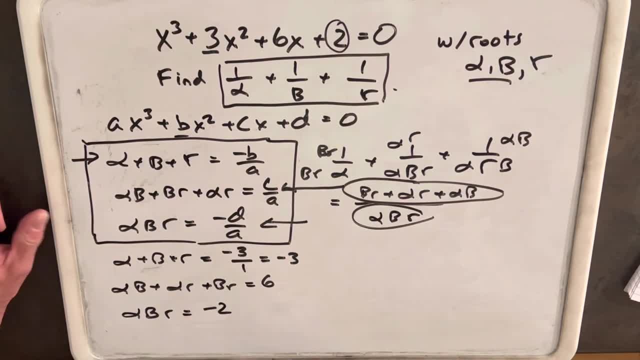 then all we need to do to finish this off is we need to plug our six in here and our minus two in here, and then we can solve. so we'll have the sum of the roots by two. at a time is going to be. 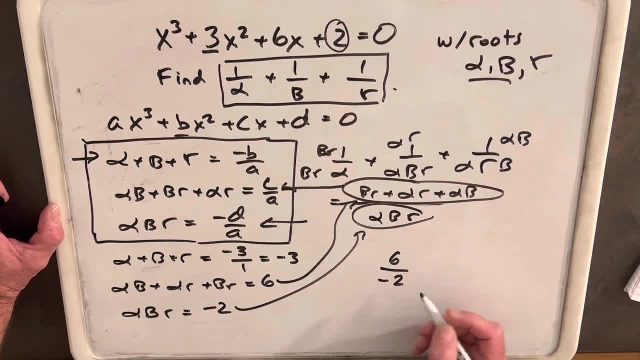 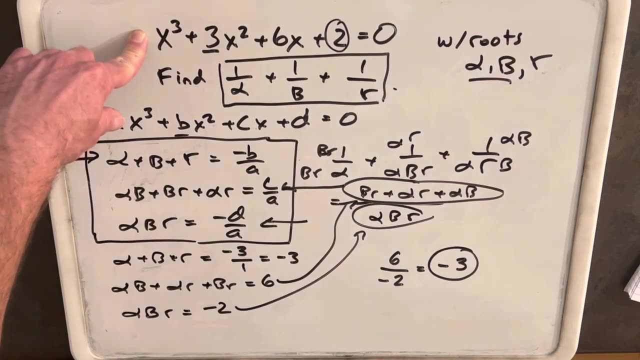 six over the product of the roots is minus two and that's just going to reduce to minus three. i did look into it briefly to try to solve this by other methods, by trying to use, like the quad, not the quadratic formula, but try to find the roots. there is one real root to this and two. 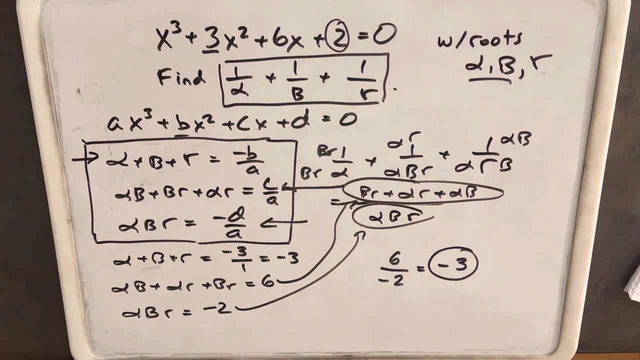 complex roots, but they were actually really messy. i think it actually would be much more difficult to try to find these three roots independently and then solve it that way. i think would be a much longer problem. so i think this is a case where vieta's formula is easier. i got this problem from 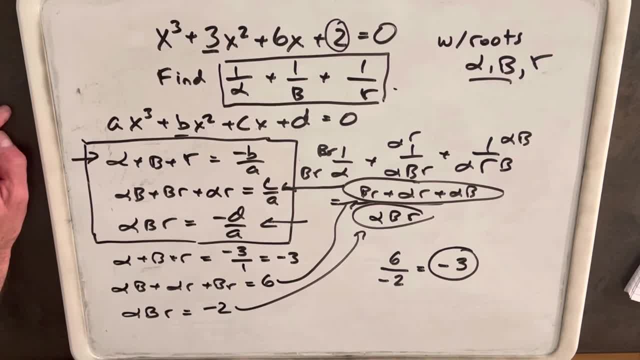 my quiz, vieta's challenge, on my website. i'll post a link in the description. i hope you check it out and i'll see you in the next video.